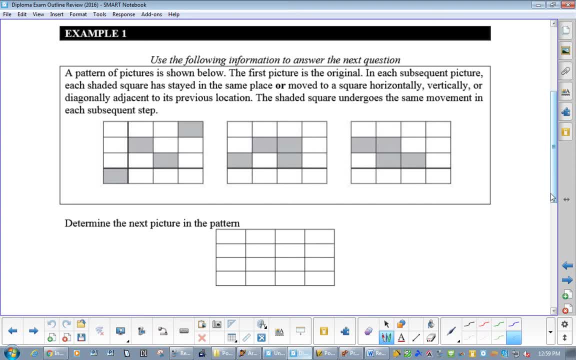 You're just already done. Oh, you're just showing me the answer. Okay, Well, I see that this one has moved up to here. You see that? And I see this one has moved this way to there And the other two remain. These did not move. So in the next picture, this one goes up, So the last one goes up. 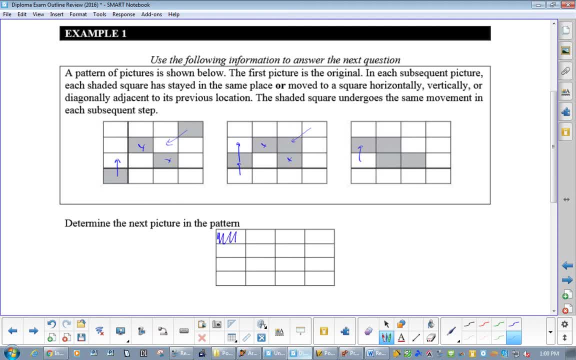 This one. this one should be here Now. these two, remember, did not move. This one started here, then went to here, then went to here. so the last one should be here. Okay, So that would be our fourth picture. Make sense. 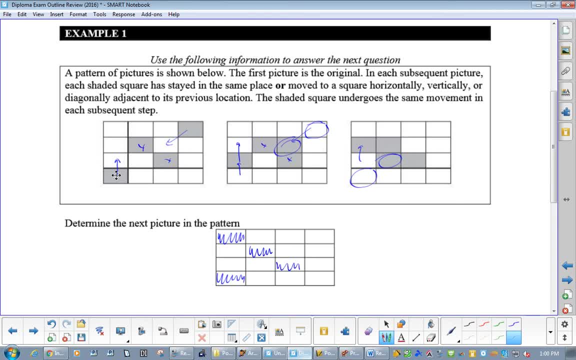 Again, just to have seen it once. So when you get the same one on the diploma, it seems familiar Like they'll mess with what the squares are doing. But they're not going to be here, They're going to be here. 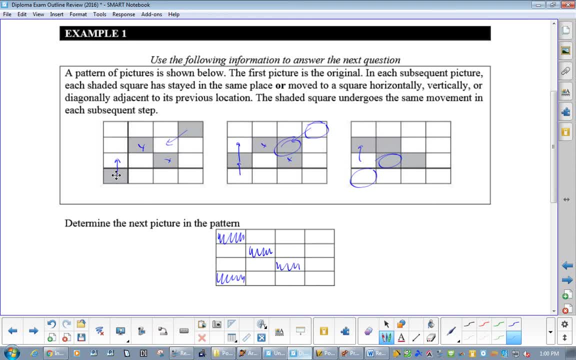 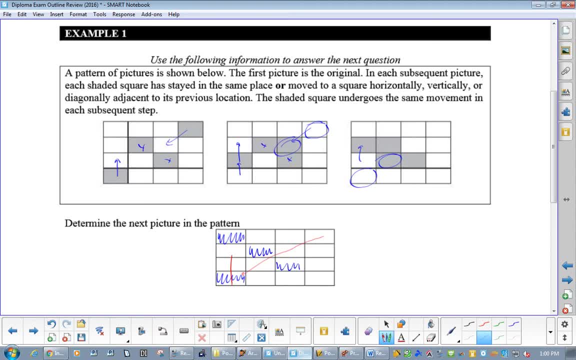 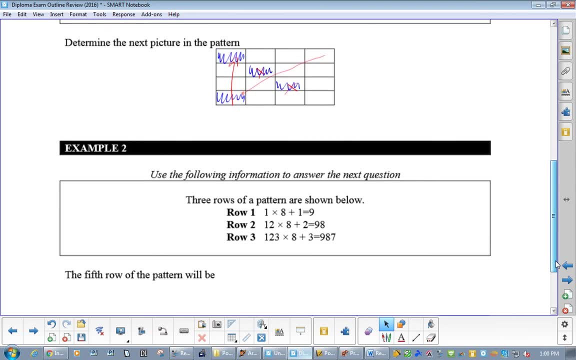 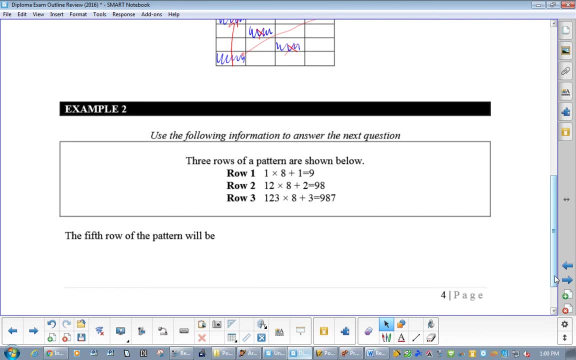 This one came all the way down from there and this one came all the way from there, And these two stayed the same. Okay, Next one. We've got 1 plus 8 plus 1 equals 9.. Then we've got 12, or times 8,, I should say. 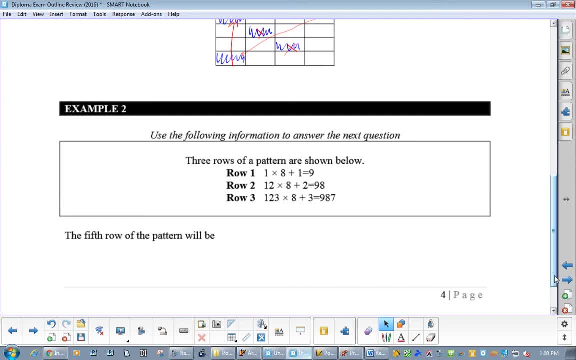 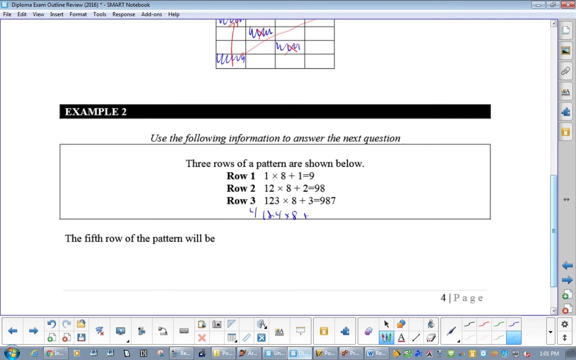 12 times 8 plus 2 equals 98.. 123 times 8. Plus 3 equals 897.. Okay Now, what would row 4 be? So 124 times 8 plus 4. And this equals 9876.. 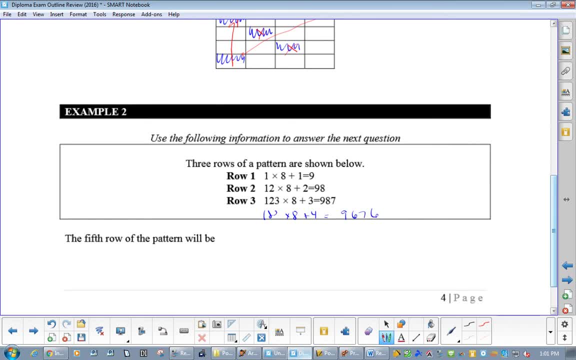 Yep, Yeah, I did, I did Okay. And then the next one would 1 be 1.. 2,, 3,, 4, 5 times 8 plus 5 is 9,, 8,, 7,, 6,, 5.. 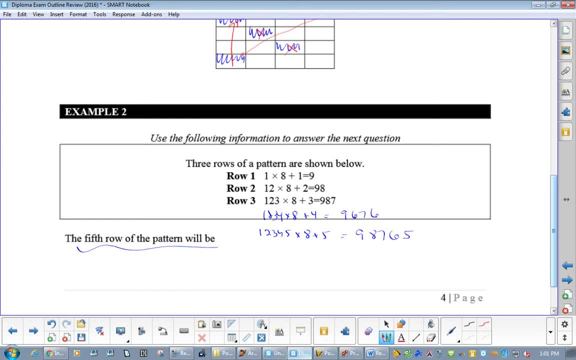 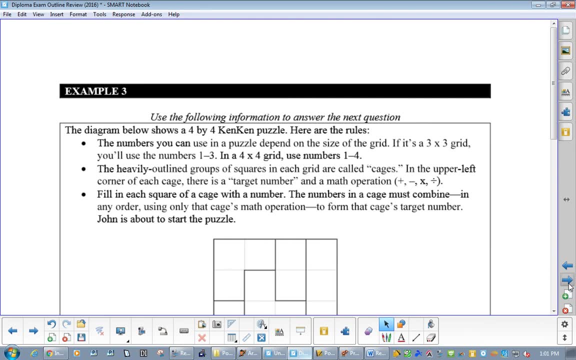 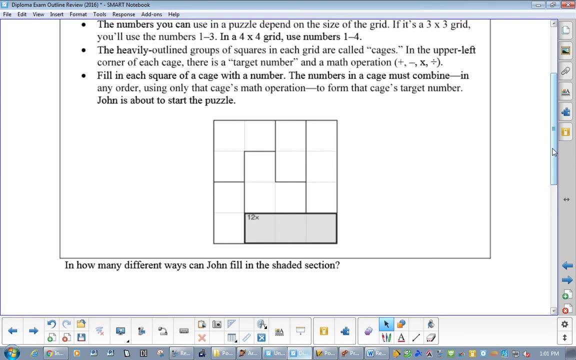 Okay, Okay, remember we did these Okay, and I don't know how well yours photocopied. but there is these light little lines, right? So maybe just draw them in really lightly, because it kind of looks like they're rectangles, right? 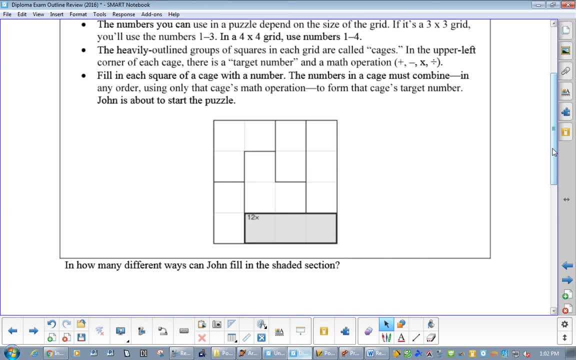 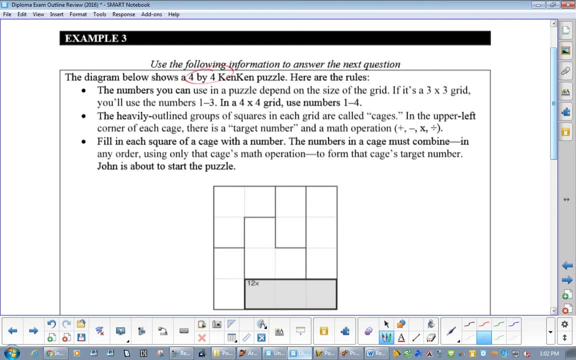 But they're not. They're all squares. Now the numbers. so this is a 4 by 4.. Okay, Now for a 4 by 4, you can only use the numbers 1,, 2,, 3, and 4.. 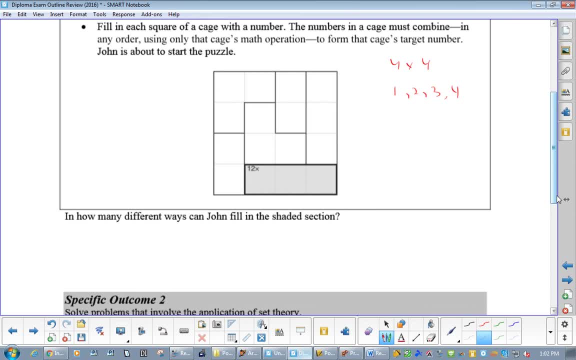 And it asks: how many different ways could John fill this in? Okay, Okay, so first of all, what times? what times? what equals 12? 1 times 4 times 3.. 1 times 3 times 4.. Okay, so, 1 times 3,. we already did. 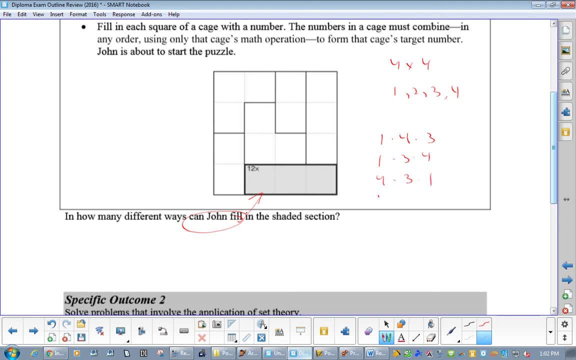 So 4 times 3 times 1.. 4 times 1 times 3.. 3 times 4 times 1. And 3 times 1 times 4.. Am I missing any? This is the same thing. There's 3 numbers. 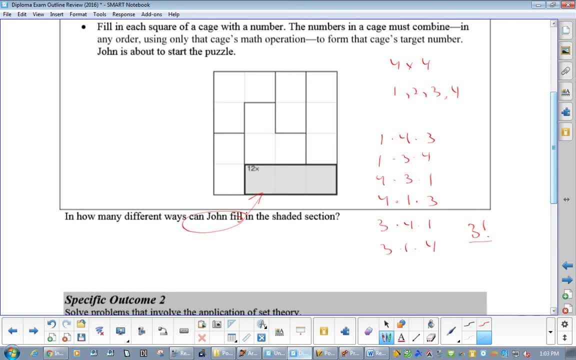 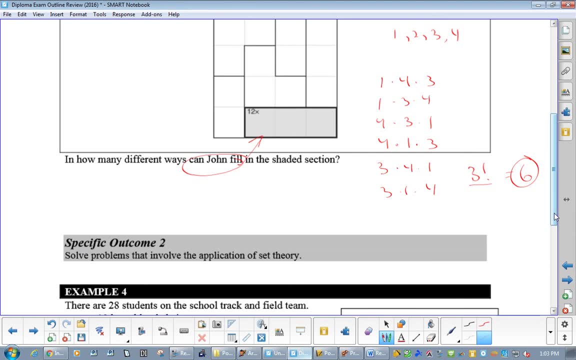 The same thing as 3 factorial, 3 times 2 times 1, right, But you will get 6 ways. So again a numerical response question You just put in the 6. Here's where they're going to get you, though. 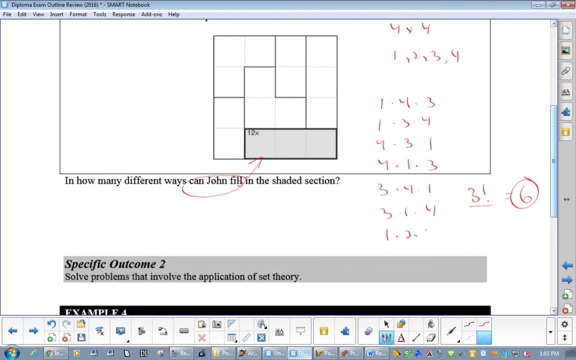 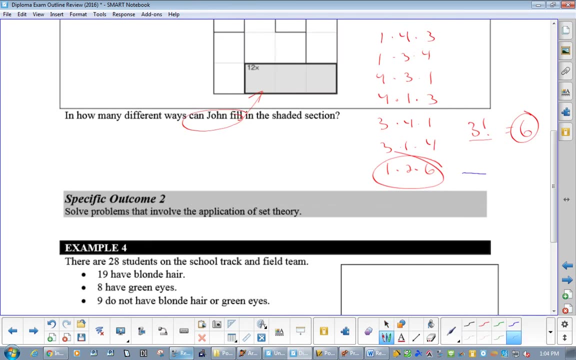 It's because people are going to try 1 times 2 times 6.. Scott, please excuse this interruption. So this is the problem: 1 times 2 times 6, people will try Because they do multiply to 12.. 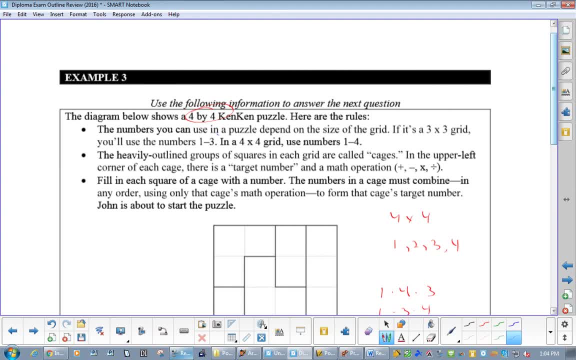 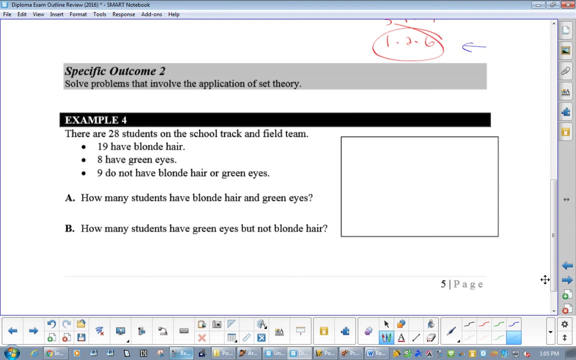 But you're not allowed to use right. You can only use the numbers 1 to 4.. So it is the common error that some students use. Okay, then we're to these. We have 28 students on the school track and field team. 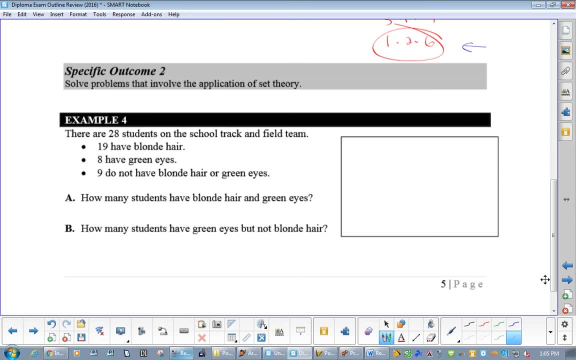 19 have blonde hair, 18 have green eyes, 9 do not have blonde hair or green eyes. How many students have blonde hair and green eyes? So what are we looking for? What are we looking for? We always call it the football. 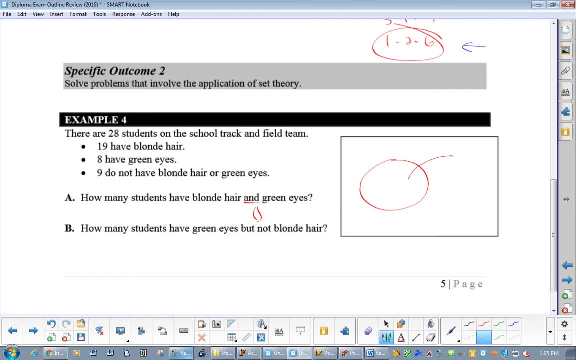 Yes, we are, So we have 2.. What are the names of the 2 circles? So we got blonde and green eyes. What are my numbers? I'm going to be putting in 19 minus football. We don't know the football, though. 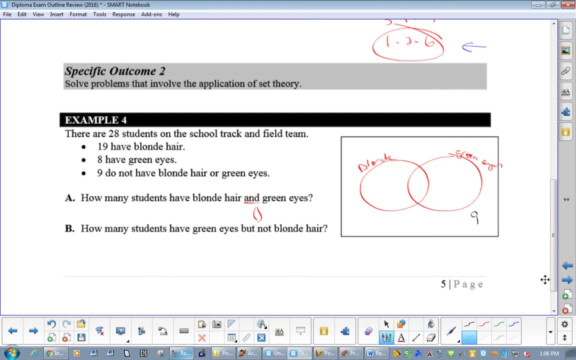 Okay, very good, We put 9 out here. That's huge. So we got: 28 minus 9 equals 19.. So 19 students have to be dispersed within the 2 circles, And this is key 9.. 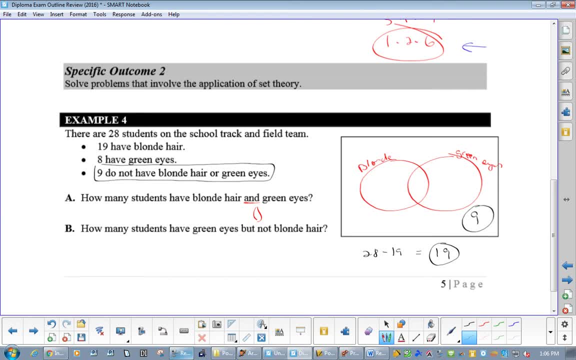 It says 9 do not belong in. Oops, 29 minus 9.. I mean 28 minus 9 is 19.. Okay, Easy, Just breathe. It's going to be okay, Okay, So now what? Okay, this entire thing has to add up to 19,, correct? 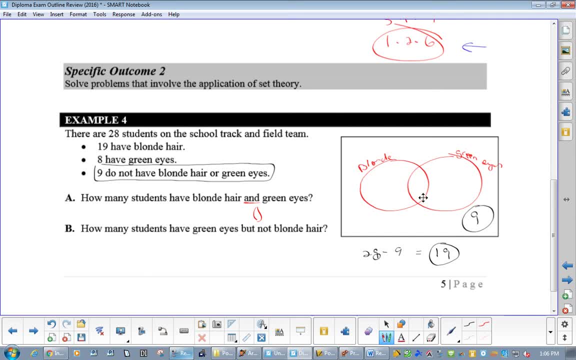 Because 19 have blonde hair, It's sterile and this It is Portable enough. So what do we minus what? It's11 minus 4 would be正 in? Yeah, You can make heavily Yeah, Maybe, how many are you in? 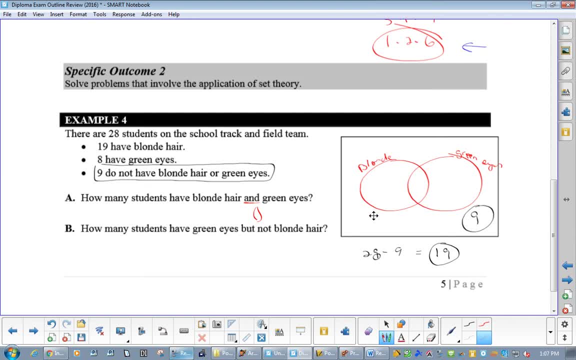 I'm sorry. The last guys are coming in out. Where are you? Okay, Kyle. Thank you. Are you there? Where is the POS code on there? Okay, Is Michael here? Yeah, He's on the POS. We're apologizing for anybody. 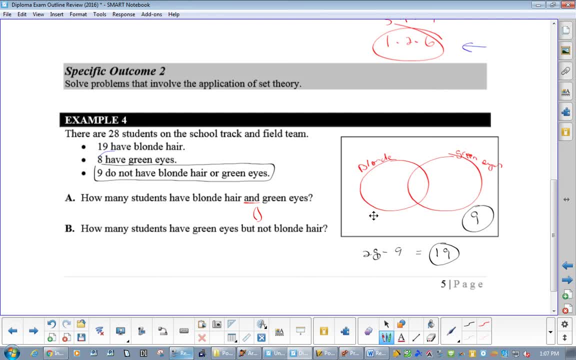 Okay, Call me. Yeah, He hasn't been here, No worries. OK. Well, first of all, Brian O' learners don't know math. He doesn't know how to manage his math. He is a quick stalker. We have: 19 plus 8 equals 27.. 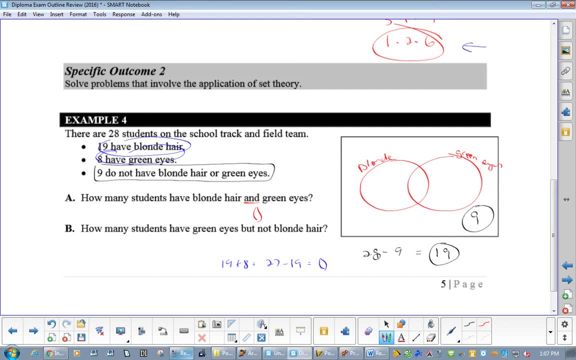 Minus 19 equals the football, and that equals 8.. So this becomes 8, and this becomes 0, and this 11.. Okay, Gordon, talk later. okay, Let's get through this. It's hot. 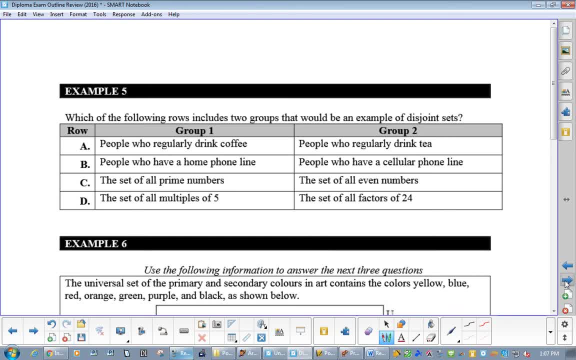 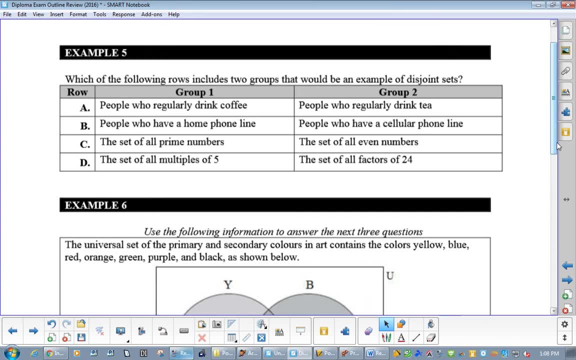 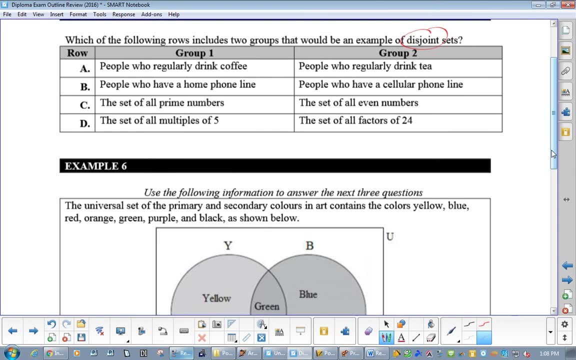 Okay, Now which of the following are disjoint? So here's a definite multiple choice. They'll ask you this because they want to know. do you even know what disjoint means? And it means that they do not have anything in common. So, people who drink coffee and tea. 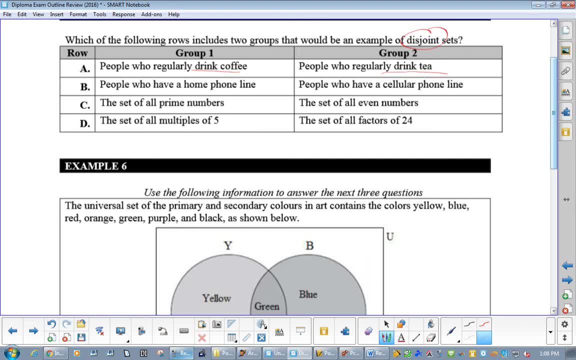 Now you have to ask yourself: can you drink coffee and tea? Yes, Next one: have a phone line and have a cell phone line. Can you have a phone line And a cell line? okay, Prime numbers and even numbers. 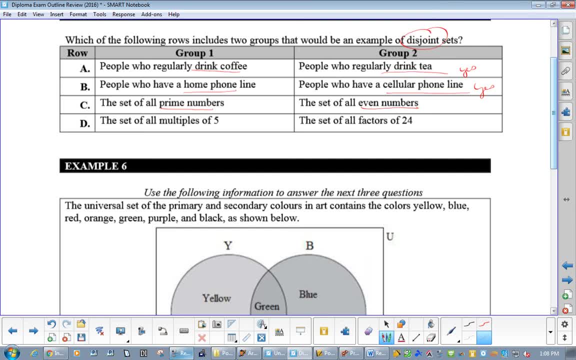 Does everyone know their primes? One is not a prime. No, you missed one. Okay, guys, people are like it's like an auction up here, So it is a number that can only be divisible by one in itself, so one doesn't count. 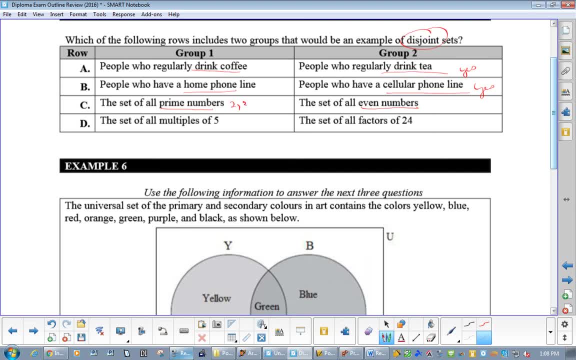 So what's the very first prime number? Two, three, five, seven. Next one, Eleven. okay, They cannot be divided. Nine can be divided by three. Now can you be prime and even Yes? What's the example? Two, Multiples of five and factors of 24.. Multiples of five, or what Five? No, you got them mixed up: Ten, 15,, 20.. What are the factors of 24? One, twenty-four, two, twelve, three, eight, four and six. 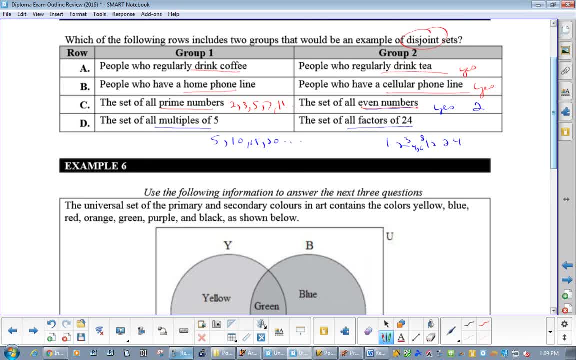 Do they share? This is disjoint. so the answer is D four six, all the multiples of 42, so one times twenty-four, two times twelve, three times eight, four times six. It is nice to know the advent of numbers, but it makes sense, even though I will think. 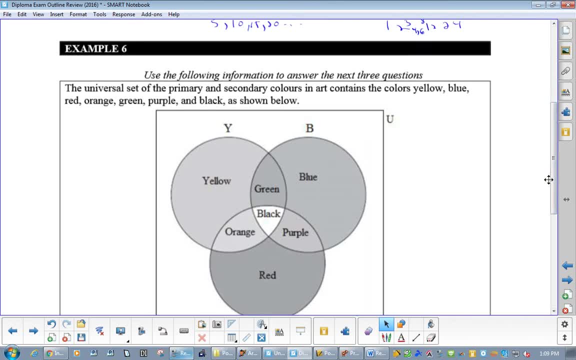 about this again next time, because we are in the memory of of what we are. So the first best fact that people say is: the universality of everything is equal to minus seven. It just means that even the opposite of the我, However, be it a part or not a part, or something. but the answer is D. you can't put in one or you cannot say it is the herb in the green. If there is an article here or something, well that piece of paper, we put it in the again. There is another favorite官, prematurely mentioned D. 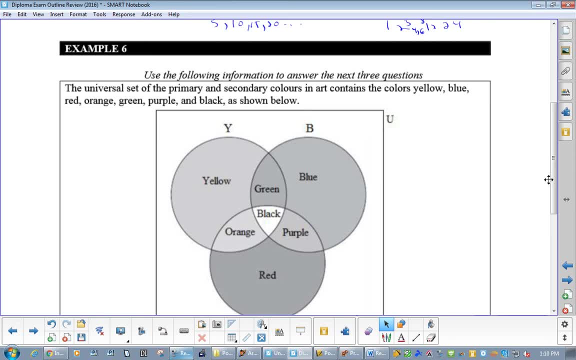 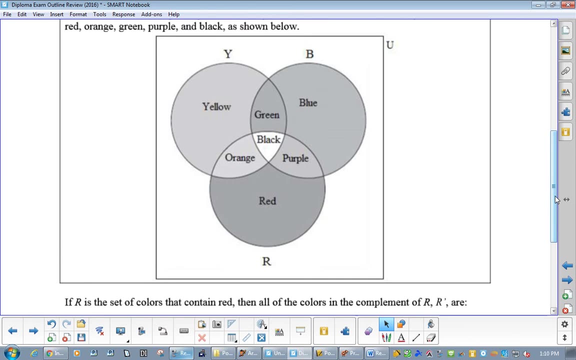 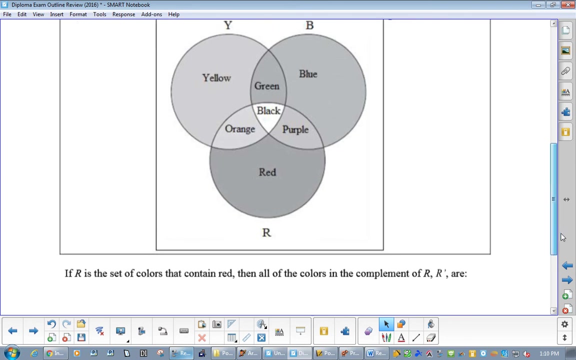 after. what he said was the things we used to make plums. That's a veryostic name. What do we say? glory or glory, If it is to be мож. In what context? is meregli guitar red then? what is the complement of R? In other words, what is R prime? This is the 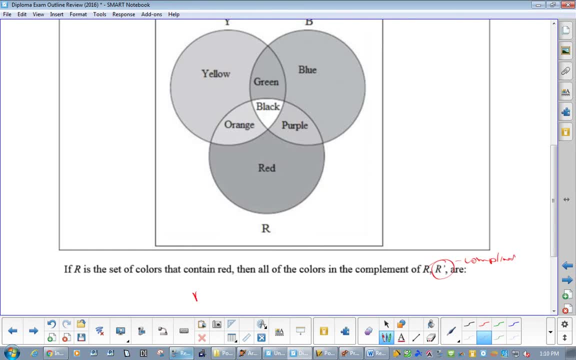 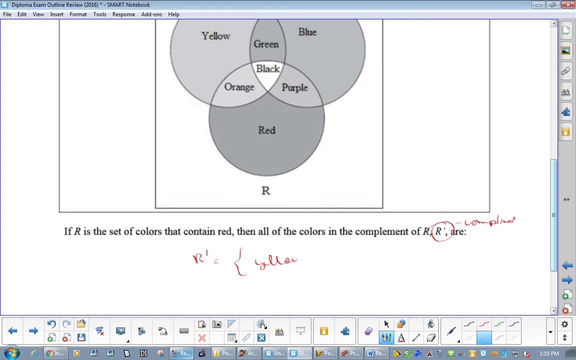 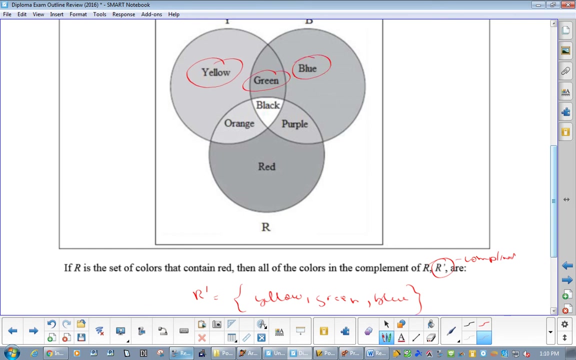 complement. So what is the opposite of yellow, green and blue? Okay, so they're the only ones that do not have red in them. Okay, so what are they asking for there? Do you know what complement means? Now, Amber. 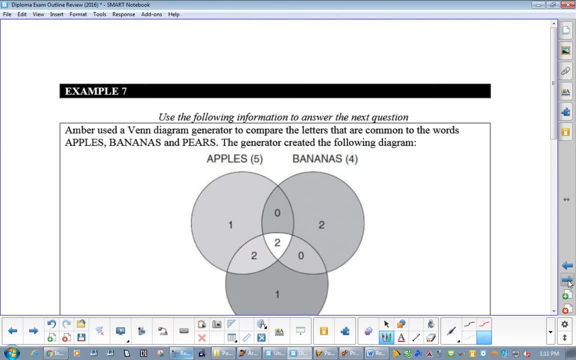 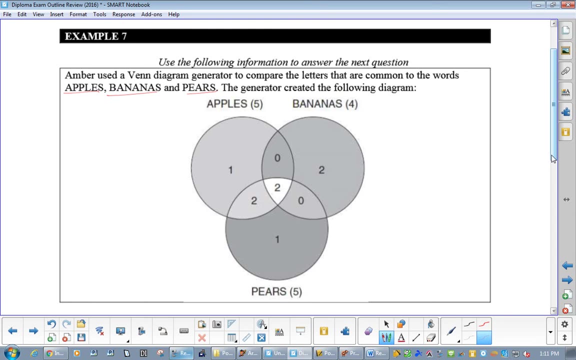 used a Venn diagram generator to compare the letters that are in common. So we got now this stuff. you really got to watch closely, right. So you got apples, bananas, pears, and they've labeled them and it says the letters that they have in common. Now the 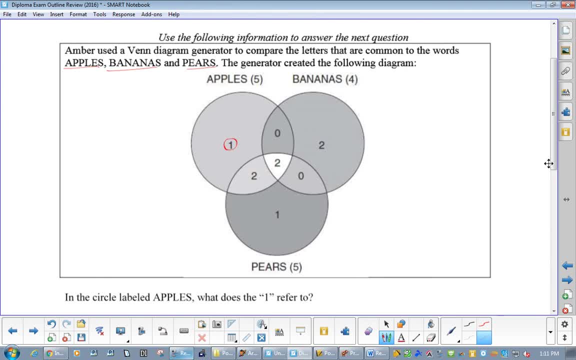 question would be: there's one letter That apples and bananas do not have in common. What is it? L Okay, banana has two letters that are not in common with anybody else. N is one of them and B Okay, how about pears? 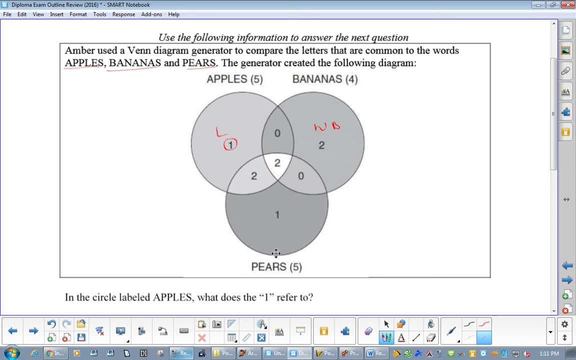 So it has nothing in common with apples, so the P would not be good And has nothing in common with bananas. R. Okay, what do you think is the two letters here? A Bananas does not have a P, S, What? 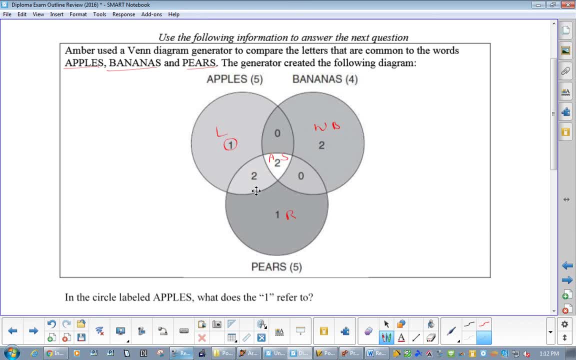 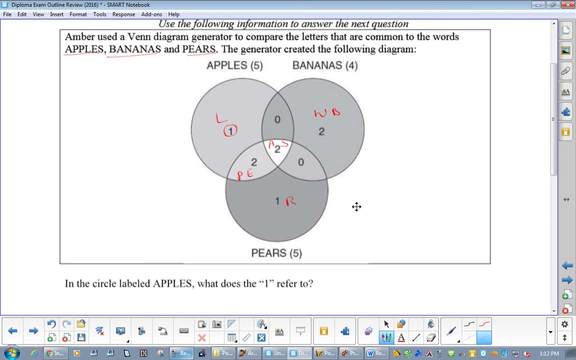 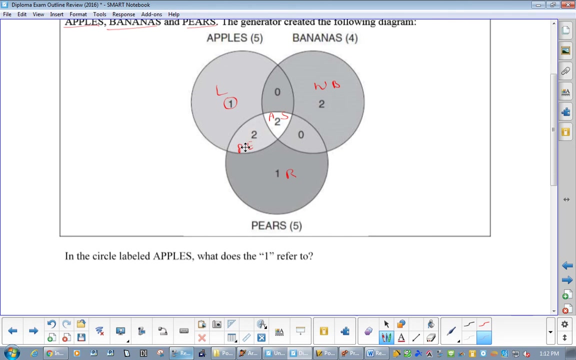 is over here: P and E. Obviously, the other ones don't have letters in them. A is in the middle, A is shared by all of them. there's two letters. So, sorry question, Yeah, they share E and they share P. They share two letters. So, Yousef, please don't. 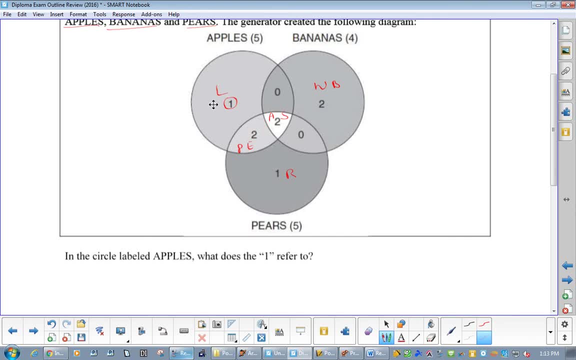 okay, This is. this is hard when people are talking, So I'd ask: what is the one R One S One R One S One A One? what is the one referred to? it refers to the L, that is, the one that Apple has. 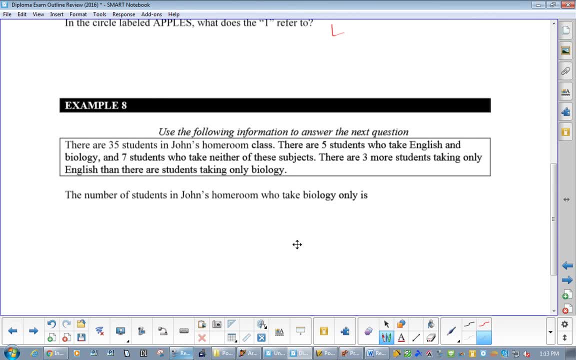 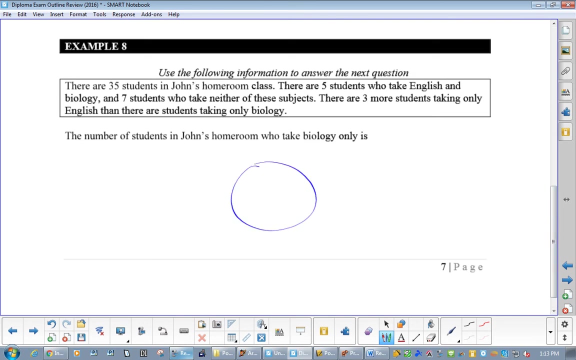 that the other one. none of this rest you? okay, there are 35 students in John's homeroom class: five students who take English and biology, seven students who neither take these subjects. there are three more students taking only English than taking only biology, so we've got our two circles. let's call this English. 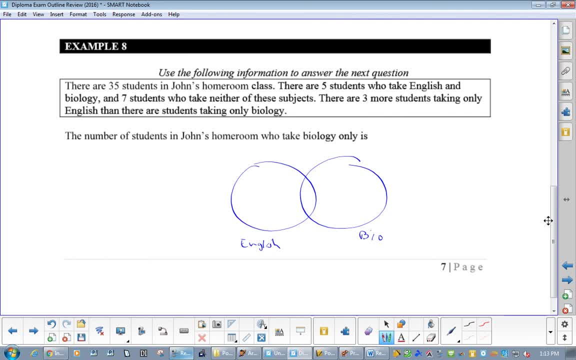 and that bio. now, remember, we are starting with 35 students minus seven, so there's seven out here. okay, good, so well, actually, yeah, okay. so so we've got 35 minus seven, that's our 28, so 28 have to be dispersed in there. how are we going to do that? 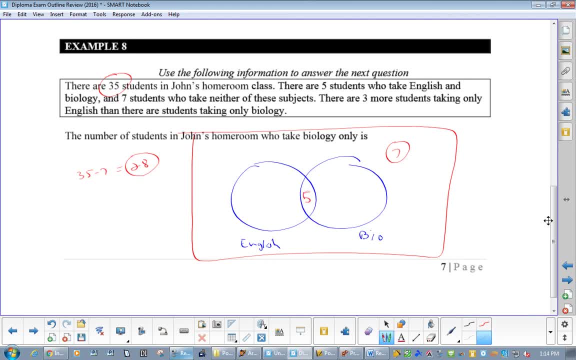 what's the football? okay, so there's three more students taking, so this all has to equal 28 and there's got to be three more in English, so 13 and 10. so the question says the number of students who take biology is 10, Only biology. 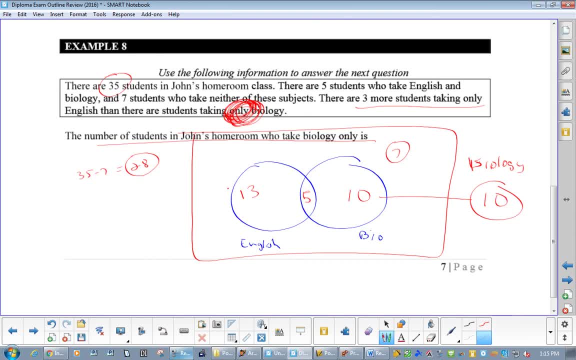 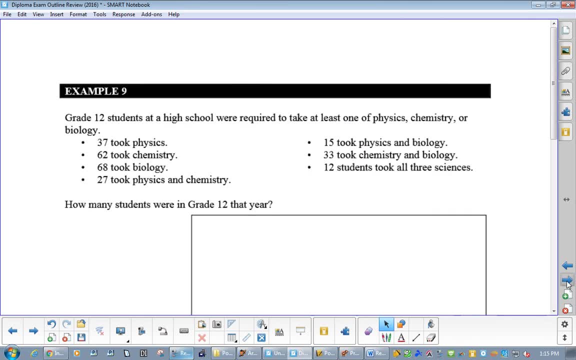 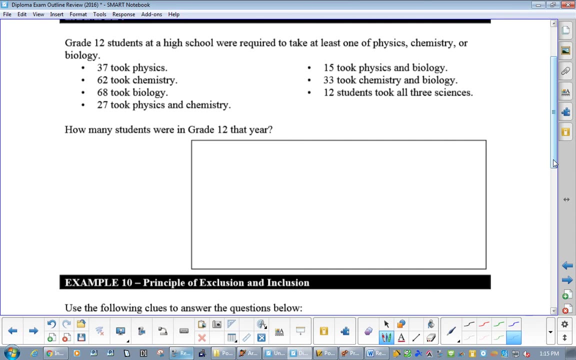 No, you just have to guess and test. This always has to be three more than that, so it all adds to 28.. Okay, Let's just get through these two. So grade 12 students in high school are required to take at least one of physics, chem or biology. 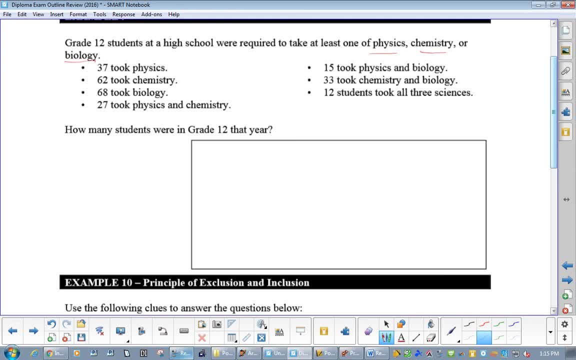 So there's no one on the outside because they have to take at least one. So we've got physics, we've got chem, and then we have bio. Okay, Okay Now. I always try to work from the 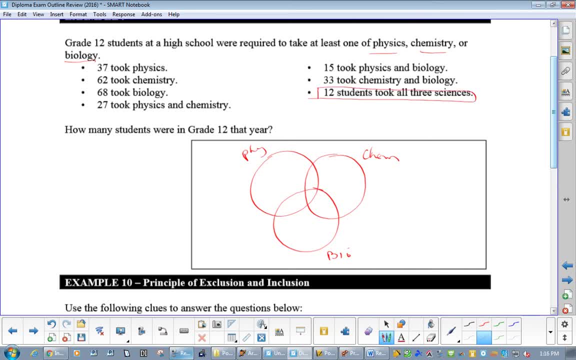 From the bottom, like this. one is our very middle, So we get the 12. students took all three. Now 33 took chem and bio, So this whole thing has to add to 33. So that's 21.. 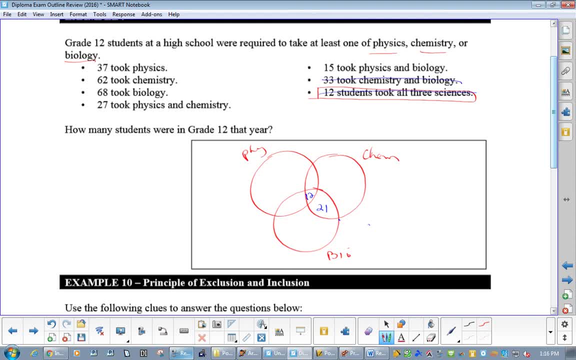 Okay, So that's gone. That's physics. took: Sorry, 15 took physics and bio, So this would be three there. 27 took physics and chem. So we've got 12 already. That's 15.. 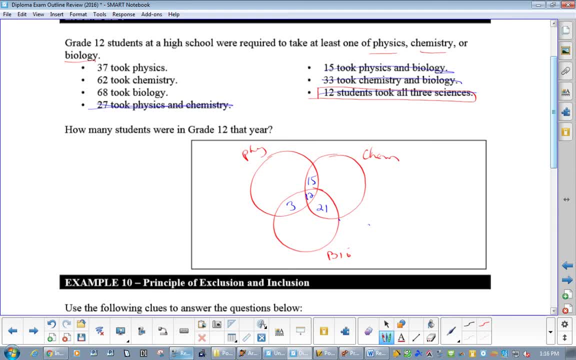 Okay, And so it's just really working backwards. Now it says: 68 took bio. So make sure that you go 68 minus 21 minus 12 minus 3.. You will get 32.. 62 took chem. 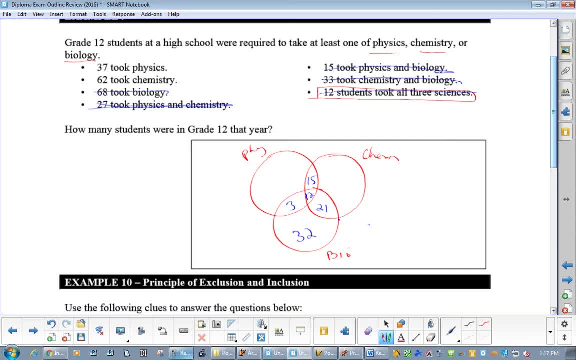 So just take 62 minus 15, minus 12 minus 20 would be 62. And 37. Oops, 14.. 14,- I mean Sometimes I get read on the next question without writing it, Okay- And 37 took physics. 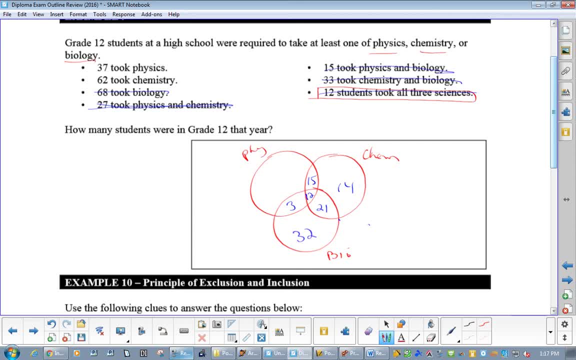 We're going to minus 15, minus 12, minus 3.. Now really We've accomplished what we need to do. It says how many students were in grade 12 that year. So very, very tough question to do without building this. 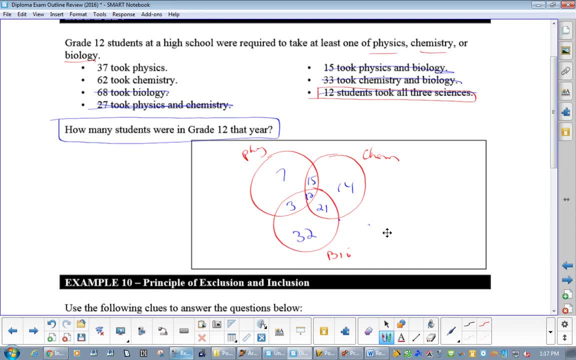 But when you have built it, just add up every single number, So Add all to get 104 students, So So. So that's a tough question, But you just go 7 plus 15 plus 12 plus 3 plus 32 plus 21 plus 14.. 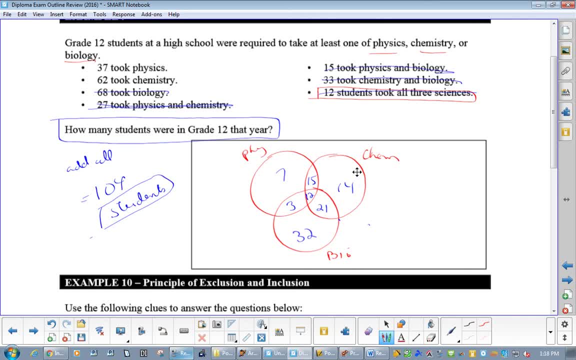 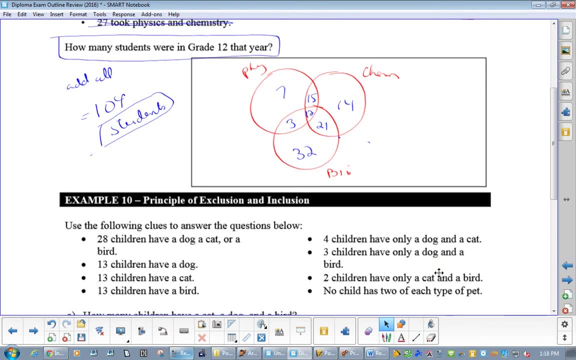 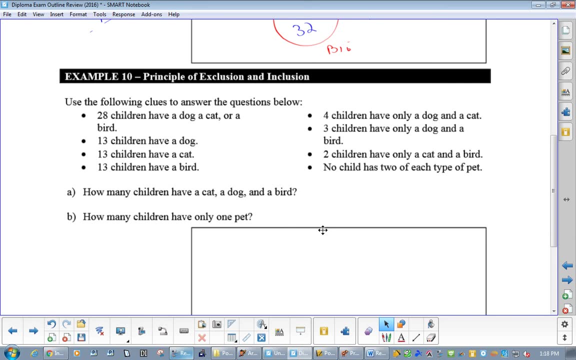 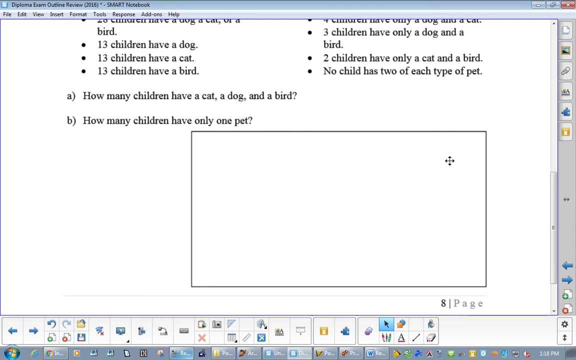 And you will get 104.. Okay, And then the last one we did was the one where you have to figure out the very center And the formula. we did that. okay. Now they will give you this, hopefully, but you have a quiz tomorrow. 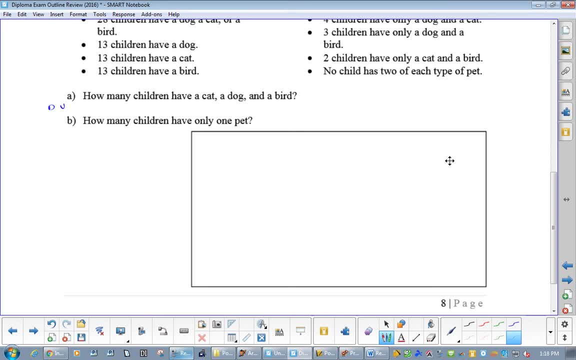 So D? U D stands for dog and cat and bird equals cat plus dog plus bird minus. oh no, that's dog or cat or bird, sorry, minus dog and cat minus bird. Okay, Dog and bird, I want to put and, but it does mean that. 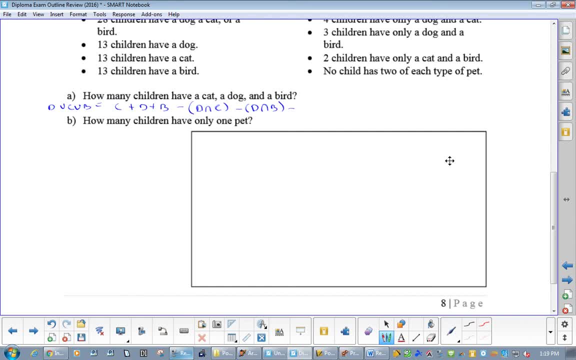 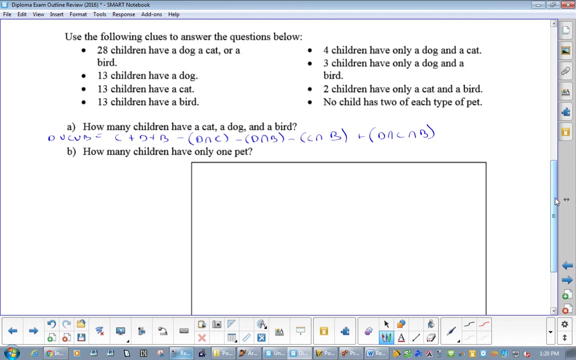 And I did it again, Minus cat and bird. Good afternoon staff, And would you please follow with a few minutes. Okay, So, as I was going here and then plus dog and cat and bird, Okay, Now it says 28- have a dog, a cat or a bird. 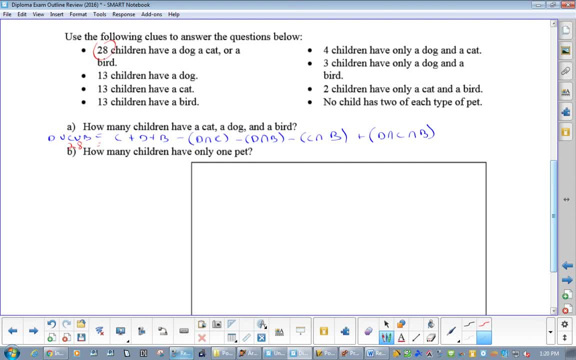 So that goes there. Equals: 13 have a dog, So that will go there. 13 have a cat And 13 have a bird- Gone, gone, gone. Four have a cat, Only a dog and a cat. 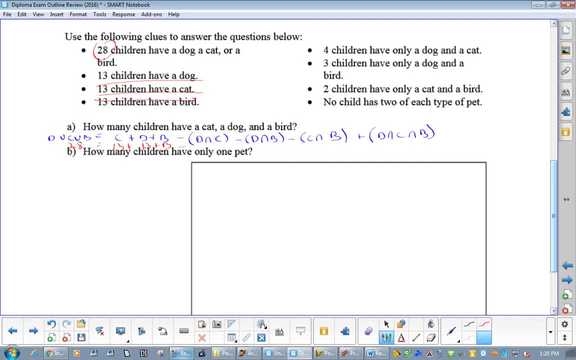 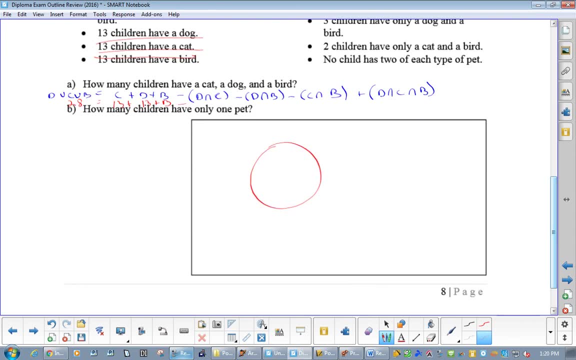 So my dog and cat is here. I'm going to go minus Now. I guess we should talk about so you get this Again. if you're not interested in this. please don't bug people that are okay. Okay. 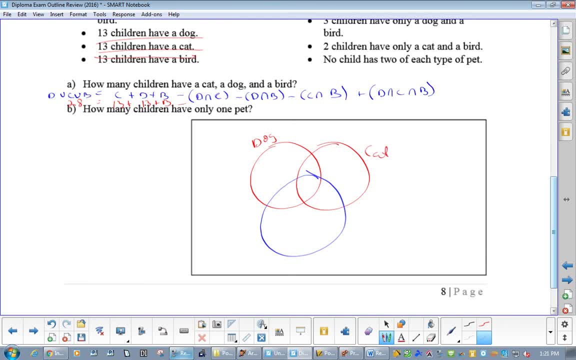 So we have dog, We have cat, We have bird And we have an X there. So four have only a cat and or dog and cat. That's four. Three have only a dog and a bird. Dog and bird is three. 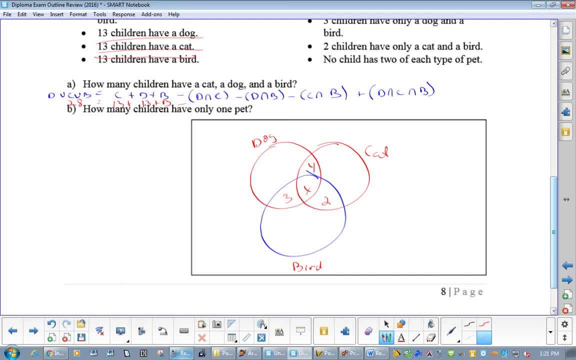 Two have only a cat and a bird, That's two. So how many people have a dog and a cat? That's just football, right? So that's four plus X. Remember, we put it in brackets: Minus dog and bird is three plus X. 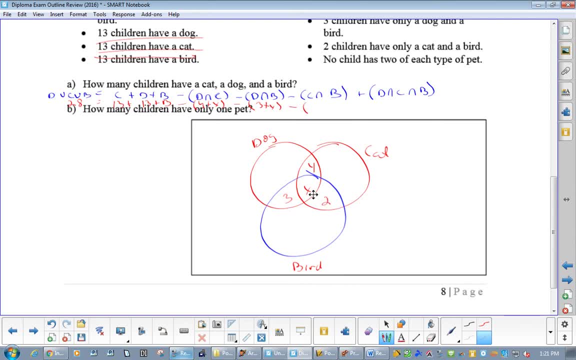 Minus cat and bird, two plus X Or X plus two, It never matters which way you do it. Plus dog and cat and bird is X. So I'm going to kind of squish it over here. but my 28 is there- equals three times 13, is 39. 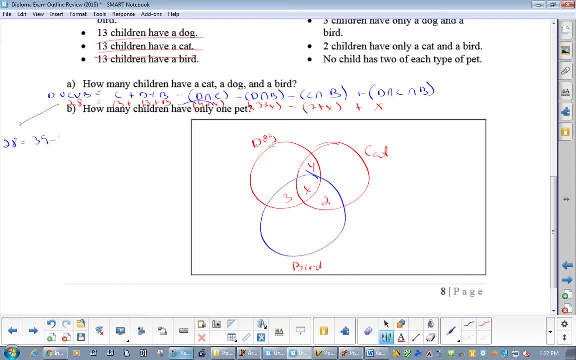 Now remember, this minus has to get distributed to here. So that's minus four minus X Minus three minus X, Minus two minus X, Then plus X Minus X. Now these two will cancel each other. 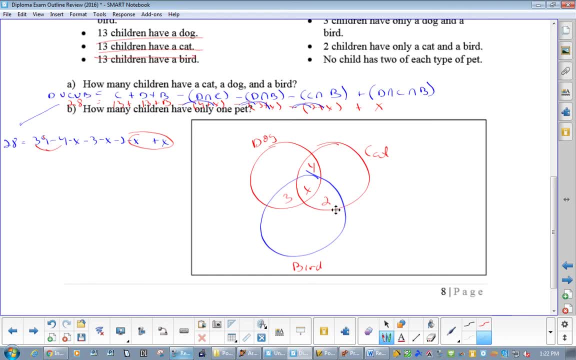 So I've got 39 minus four Minus three minus two is 30.. So I've got 28 equals 30 minus 2X. Okay, I will subtract 30 to both sides. Negative two equals negative 2X. 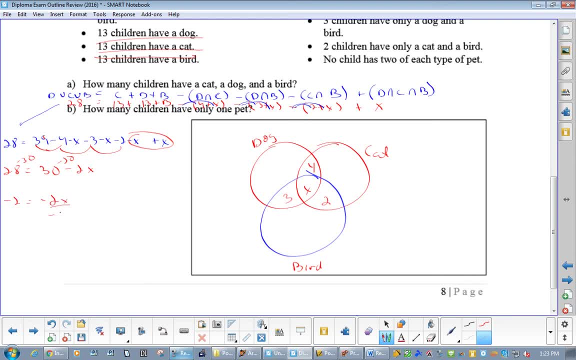 I'll divide by negative two. One equals X, So the question asks: how many children have a Good afternoon everyone At this time? we will. Okay, let's finish this. I've got another minute left, So now it says how many. 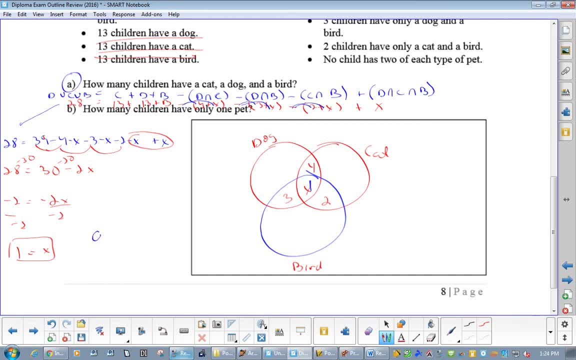 We're doing A, So that's one. now, A equals one. But here's the harder one: How many have only one pet? Well, we have. We have to go back and it says 13 have a dog. So all this must add up to 13.. 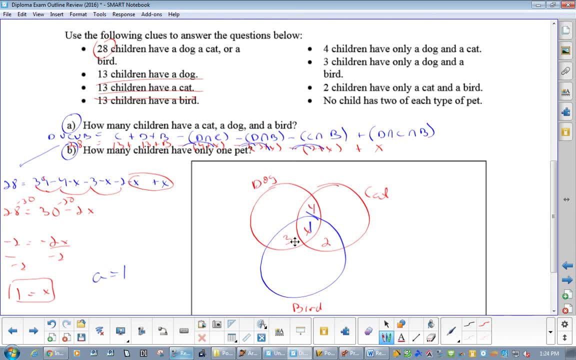 So 13 minus four, minus five, minus eight, This is five. here. 13 have a cat. So then we subtract four, one and two and you'll get six. 13 have a bird. So we minus the three, minus the one. 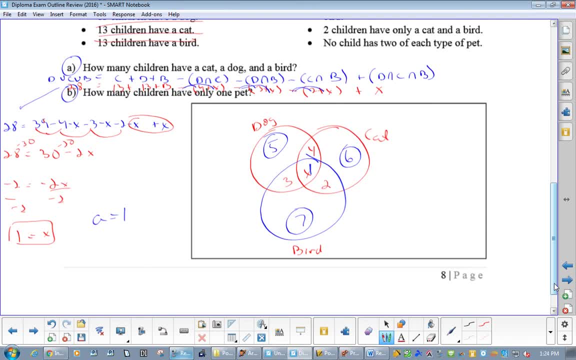 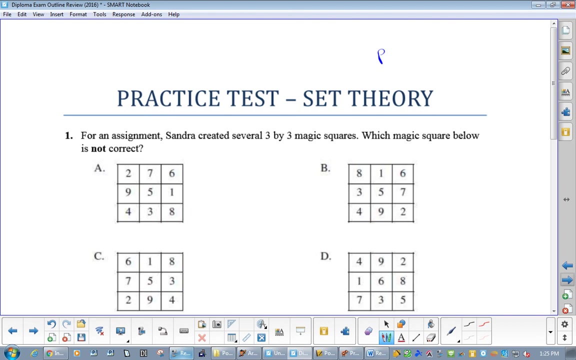 Seven. So A is one, B we have to go. Seven plus five plus six equals 18. only have one pet, Okay. so these will all be on the diploma in some shape or form. Okay, so if you turn, you're doing page nine to.